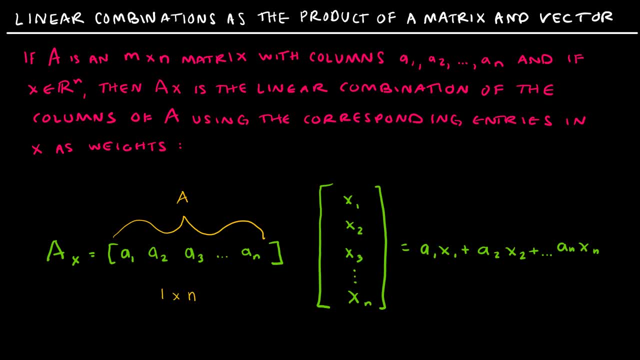 And what I'm going to do is multiply that matrix and this one again. I just did one row, but I could have as many rows as I needed times the vector that is n by 1.. So my vector is obviously going to be just one column. 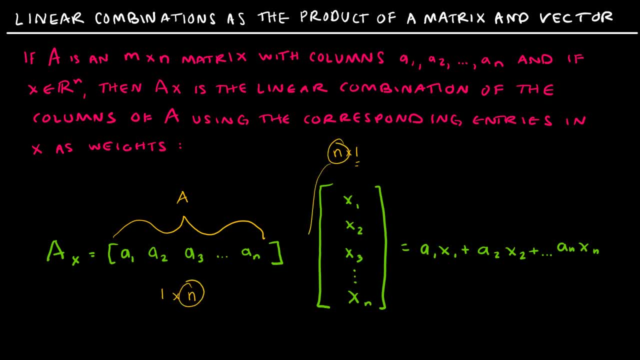 but it needs to have a, the same number of rows as A has columns, And that's where this corresponding entries is going to come in. So what's going to happen is I'm going to use these guys as weights and multiply it by everything in whichever column that corresponds to the subscript of 1,, 2, etc. 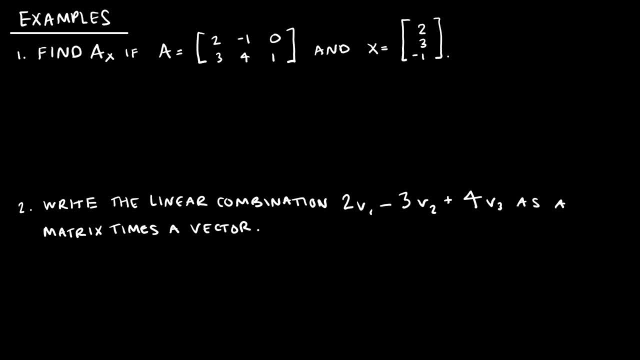 So let me show you an example. Here we're finding A times X, and they've given me A and they've given me X. So you may already know how to multiply matrices. This is not that. We're going to talk about that in a little bit. 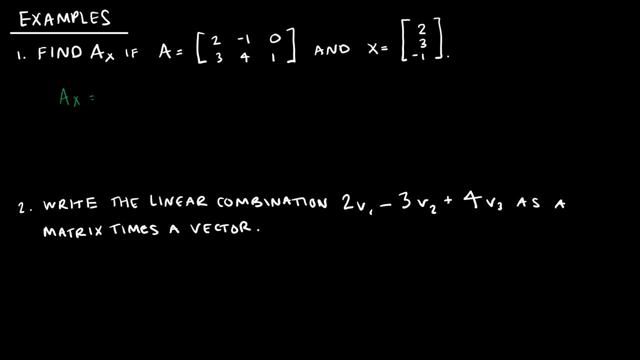 But essentially, if I'm taking A times X, I'm saying let's take 2 and multiply it by 2, 3.. So this is the first entry and this is the first column, And then I'm going to do the same. 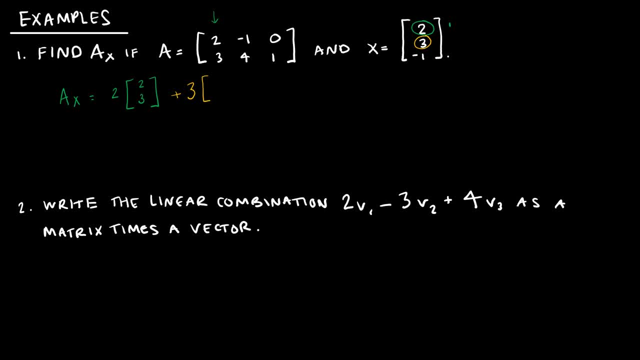 So I'm going to do the same with 3.. So 3 times negative 1,, 4.. And then I'm going to do the same with my third entry and I'm going to put minus 1, but you could put plus negative 1,. 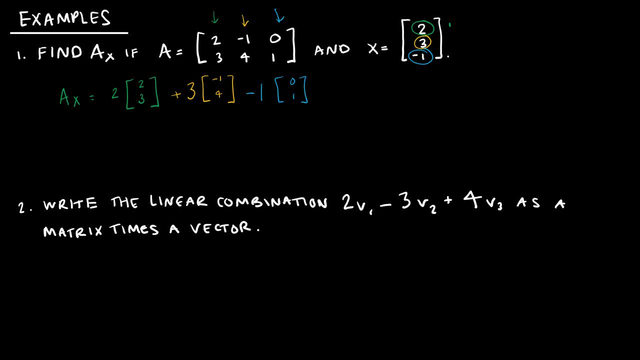 and then my third column. So then, of course, I would just go ahead and take 2 times 2 and 2 times 3.. I would take 3.. I would take 4.. I would take 3.. I would take 4.. 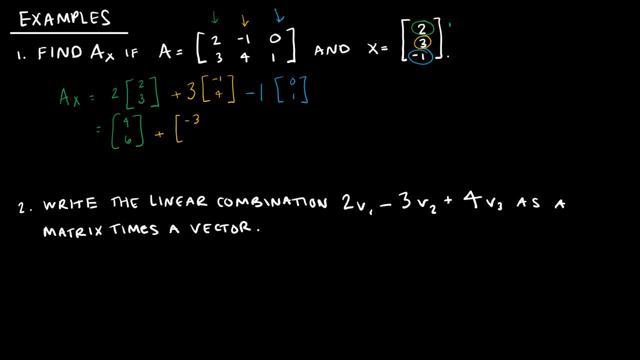 I would take 5., I would take 6., I would take 7.. 3 times negative 1, and 3 times 4, and I would take negative 1, or 1,, I guess, times 0.. 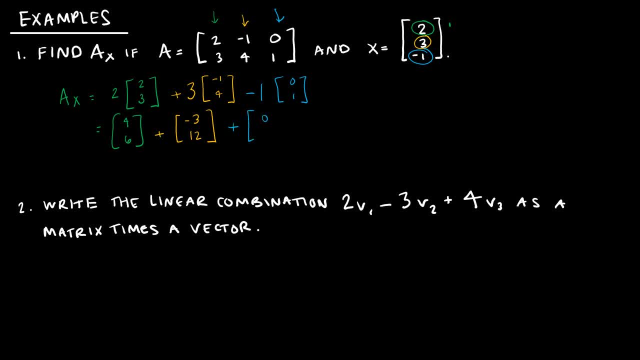 I'll just go ahead and change that to plus Negative 1 times 0, and negative 1 times 1.. And then my solution would be when I add those together, So 4 plus negative 3 is 1 plus 0,, and then 6 plus 12 is 18, plus negative 1 is 17.. 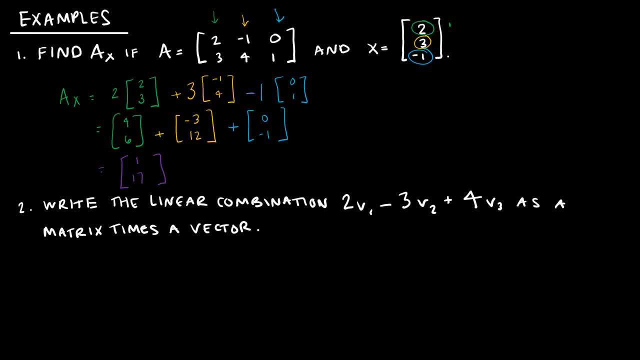 So that's pretty straightforward. For our second example, we are asked to write the linear combination as a matrix times a vector, And so this one's actually pretty easy. It looks like it might be more complicated, But essentially they're asking us to write it as a times x. 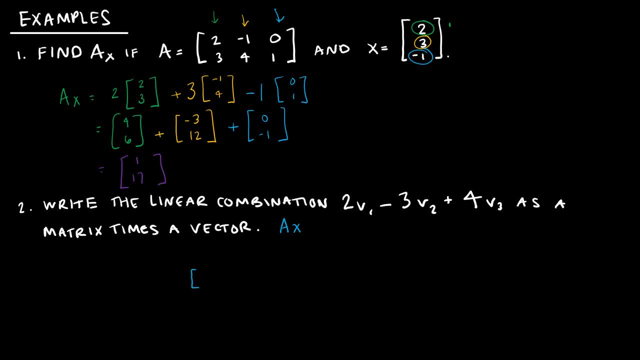 So what would a be? Well, a is going to be vector 1., Vector 2., Vector 3. And x. remember, x is the weight. so what weights am I using? 2,, negative 3, and 4.. 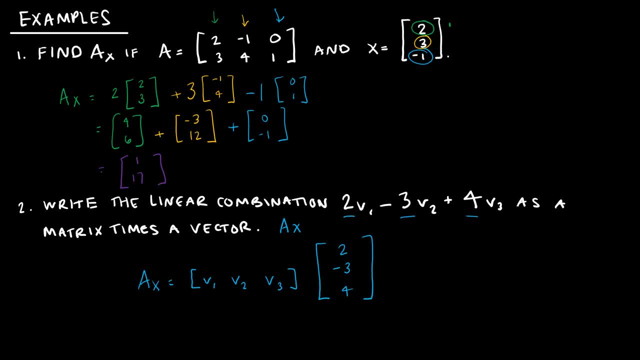 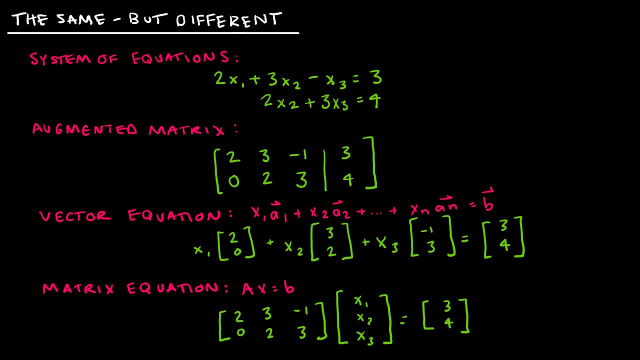 So that's all I would have to do to write that as a vector times a matrix. Before we continue through this lesson, I wanted to take a step back and make sure that you're making the proper connections. All of these representations that I have here are for the exact same system of equations. 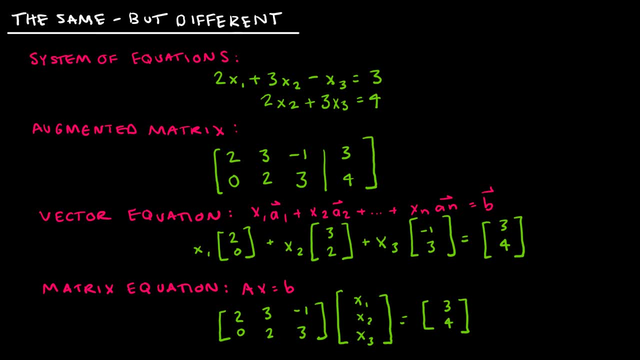 So I put the same but different, because they're the same but they are different representations. So the reason I want to point this out is so that you understand. we can write this system of equations in any of these ways and they're all equivalent. 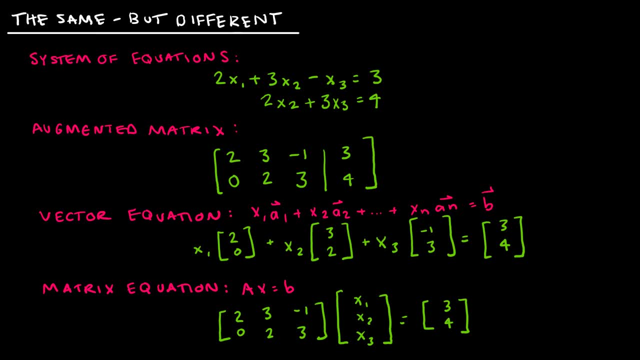 So we just need to either use what works best for us or, if this is, say, a homework question, we would use whichever representation the homework question asked for. So we'll start with just a normal system of equations. here Again, I've got x1, x2, x3, so I have three variables. 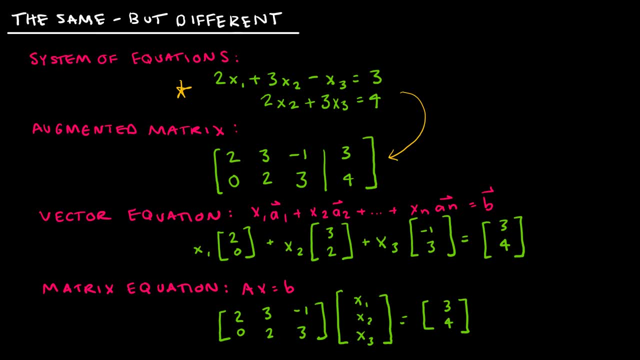 I can then write that as an augmented matrix. And again there. this side is the coefficients and this side is the solutions or the answers. Your textbook does not show this line, but I would like for you to show that line. 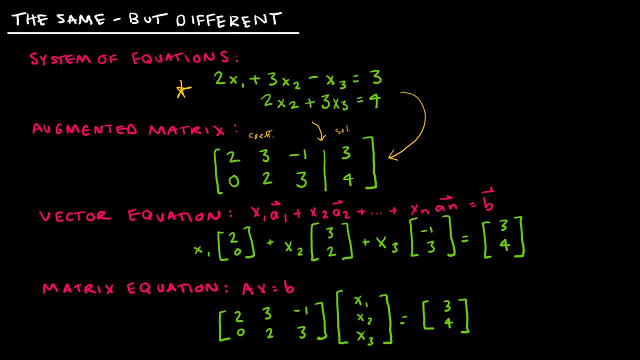 You can then write that as a vector equation. And again, the vector equation uses x1, x2, x3 as the weights times each of these vectors, And then we could also then write that as a matrix equation. So the matrix equation is what we're doing now. 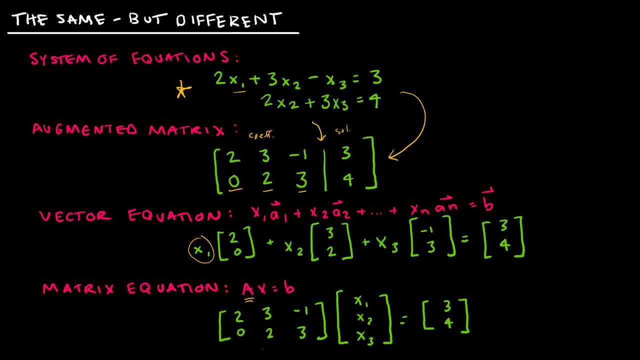 The matrix equation. as we can see, A is going to be the coefficient matrix, So it's everything And the augmented matrix that would be on the left side, that would be multiplied by our vector that has the variables. And then, of course, our solutions are here. 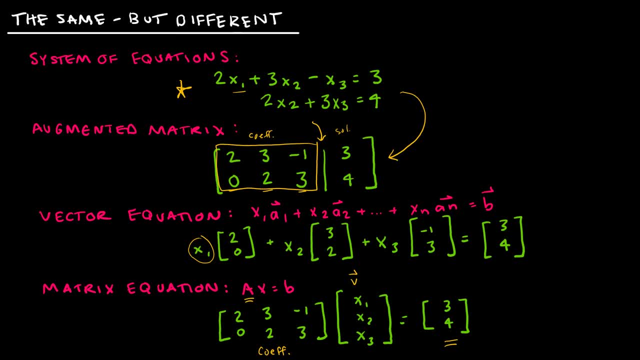 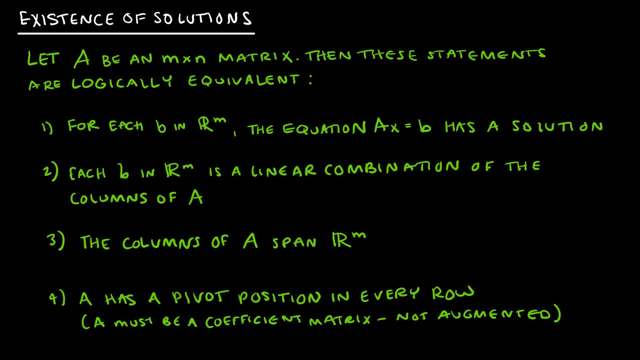 So all of these are the same system of equations, They just look a little bit different. I have one more practice I would like to do with you, But before I do that, I want to talk to you about these four statements that are logically equivalent. 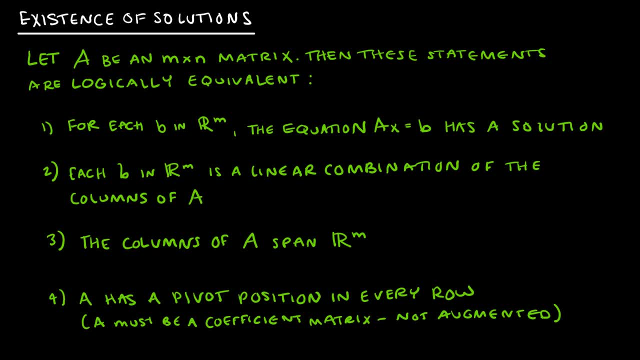 And the reason I want to point out- point this out- is because up to this point, when we've looked at solving a matrix, for the most part we had one solution, So it was a consistent system with one exact solution. Sometimes we had a consistent system with infinitely many solutions, and that's kind of what we're looking at here. 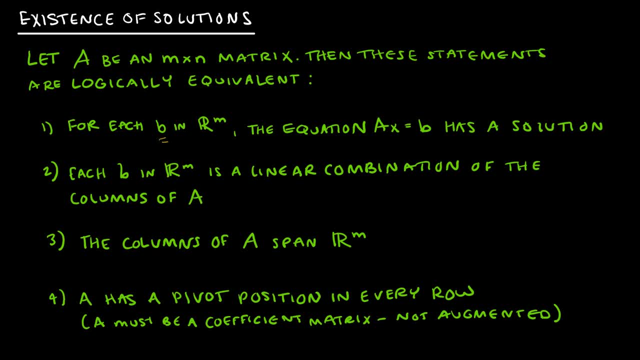 We're saying for each b in Rm, the equation Ax equals b has a solution, which means there is a solution for every b. That is the exact same thing as saying each b in Rm is a linear combination of the columns of A. So again we can take x1- A1 plus x2- A2, I might have mixed the order on those. 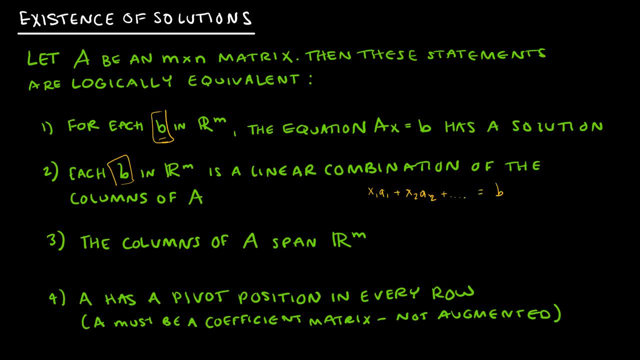 plus blah, blah, blah blah equals b, and we're saying each one of those has a solution. We of course can use that word span, which is the collection of all of the solutions, So the columns of A span, Rm. Or we can say that: 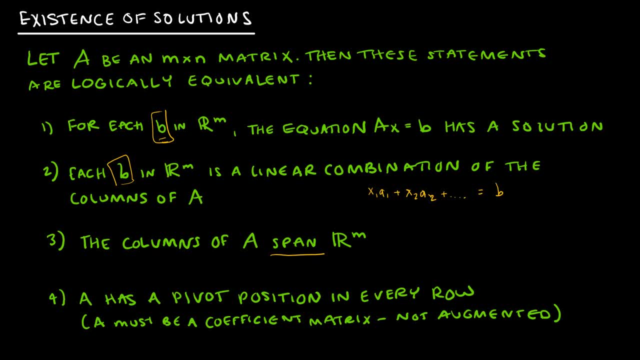 A has a pivot position in every row. And again, this is if it's a coefficient matrix, not an augmented matrix, because then we might get into a situation where we have our pivot here on the right side And of course that would mean no solution. So if we were talking about a coefficient matrix, not an, 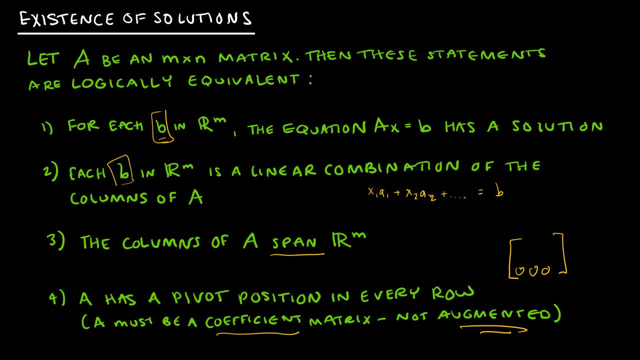 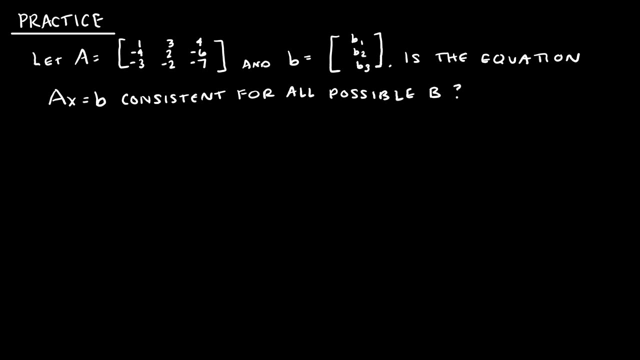 augmented matrix, then that statement is true. Now, the reason I bring that up is because on our next example we're going to look at, do we have a solution for each b? So again, this practice is looking at whether our system is consistent for all possible values, and we're 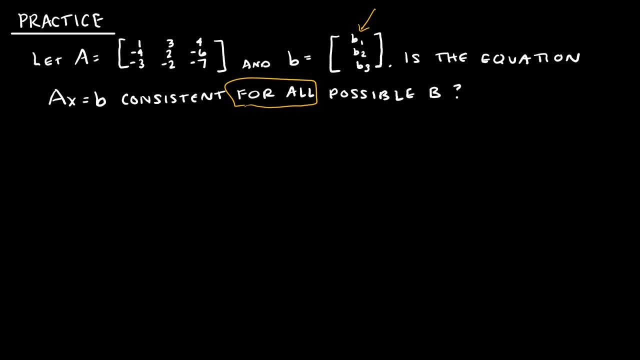 going to start saying that it is consistent for each b And again, I'm going to run this into a matrix And we're going to have now what I'm going to write here as. so I'm going to write this as a matrix. this is going to be the matrix of B and, if you'll notice, that's very clear from our matrix B. 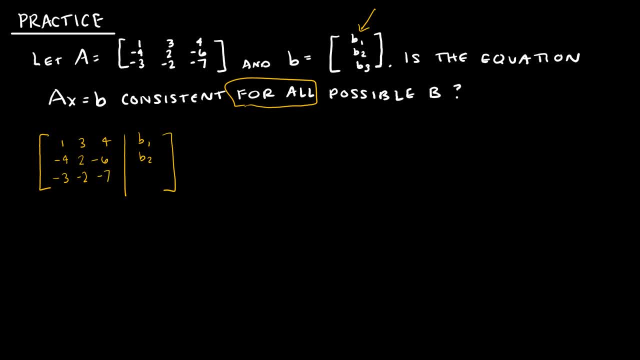 to be that b vector, oops, b3. from here i'm going to obviously do some row reduction so i have that pivot of one right where i want it to be. so my first row is looking pretty good, just as is row two. i'm going to do both in the same step, so i'm going to take negative- i'm sorry, positive- four. 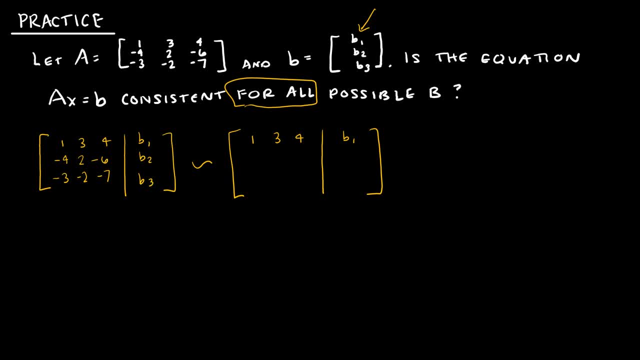 times row one and add it to row two to be my new row two. so that's going to give me zero, which is of course why i did it: 14, 10 and then b2 plus 4 b1, and then i'm going to take three times row one. 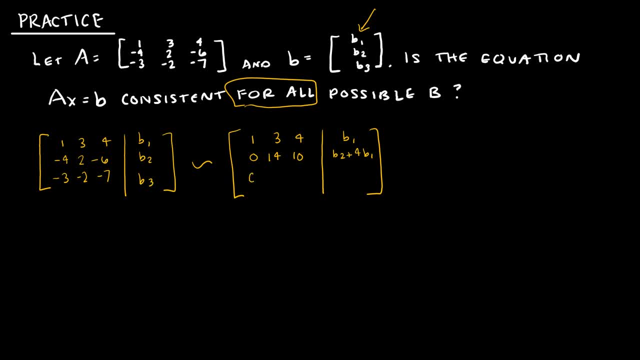 and add it to row three, so that i can make this value a zero, which gives me seven. five, and then b3 plus 3: b1, so far, so good. now, looking at my rows, it looks like 14 is going to be a pivot, so i'm 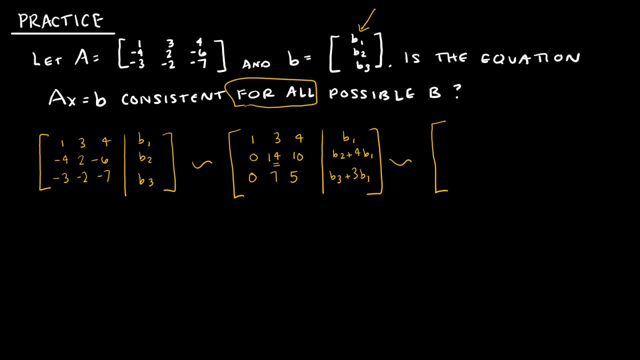 want to, even though I'd really like that to be a 1,. I really don't want to deal with those fractions right now, So I'm going to focus on making the 7 into a 0, and I'm going to do that. 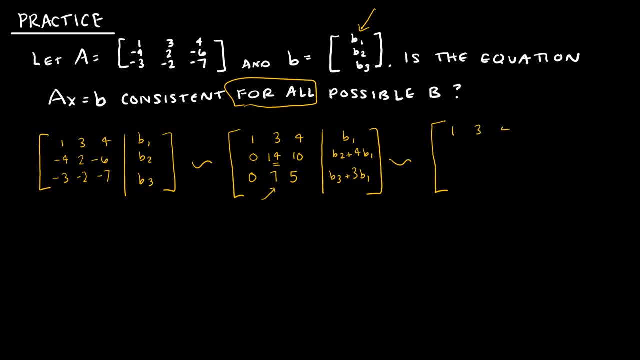 by taking row 1 and keeping it exactly the same, row 2 and keeping it exactly the same, and then row 3 is going to be negative: 1 half of row 2 plus row 3, which is going to give me 0.